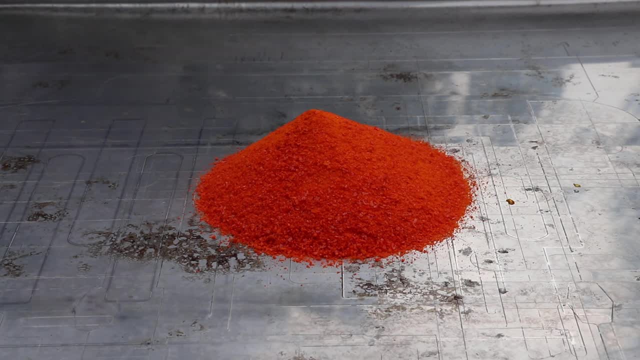 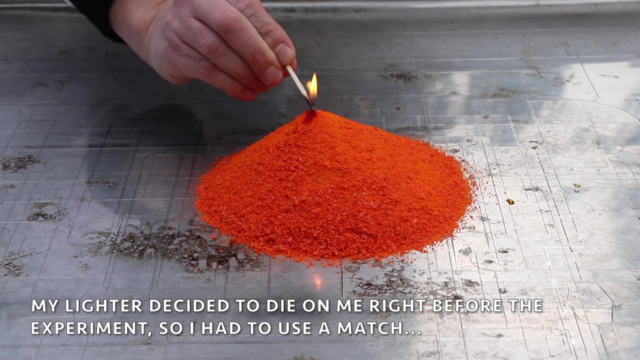 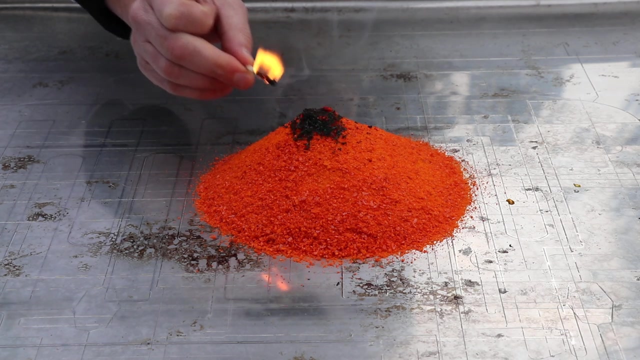 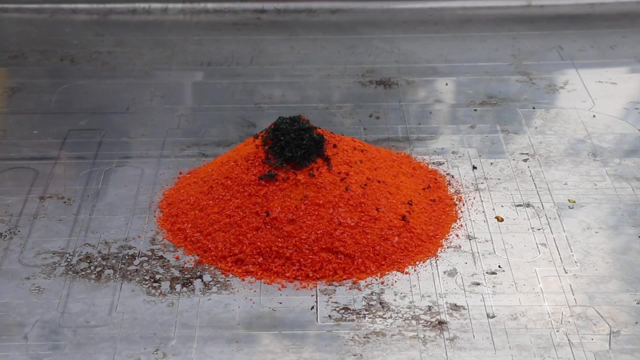 Just trying to make like a little hill like that. Now I'm going to set this thing on fire and see what happens. Don't try this at home, guys. It didn't work first time. it was probably not enough fire. Well, let's do it again. 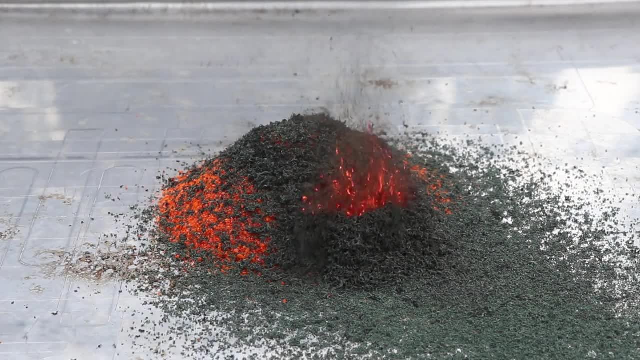 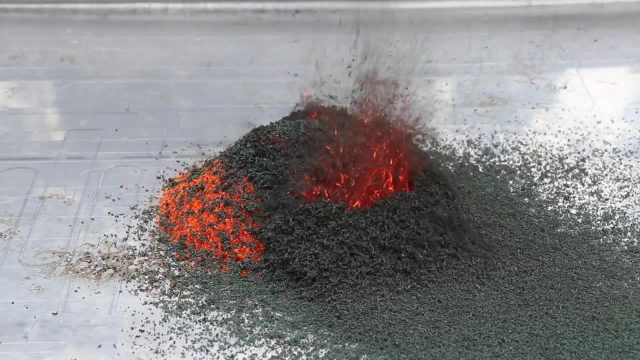 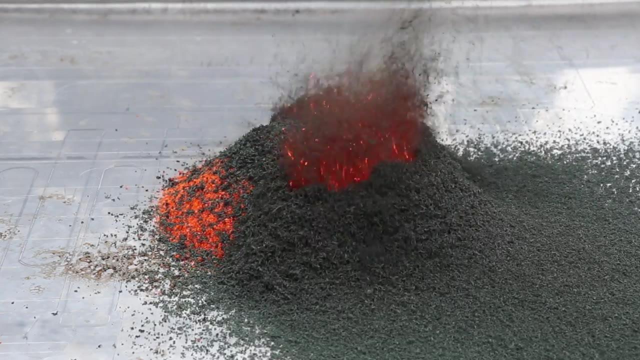 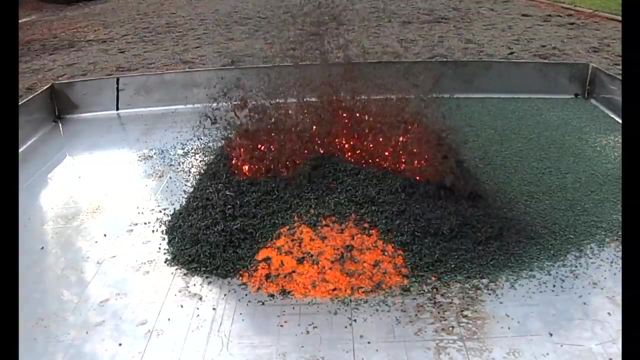 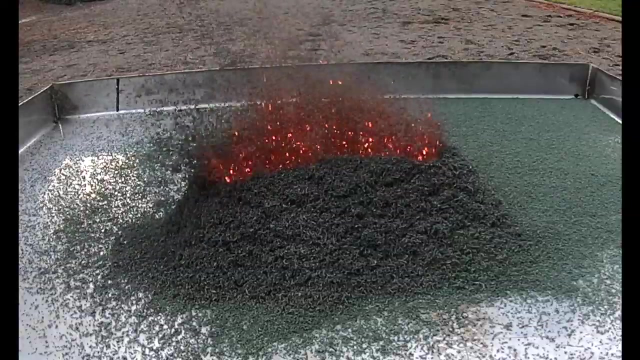 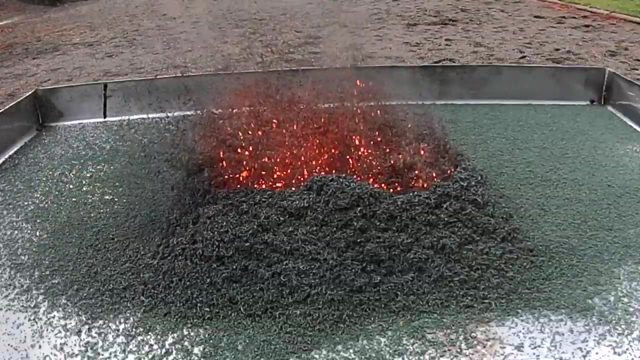 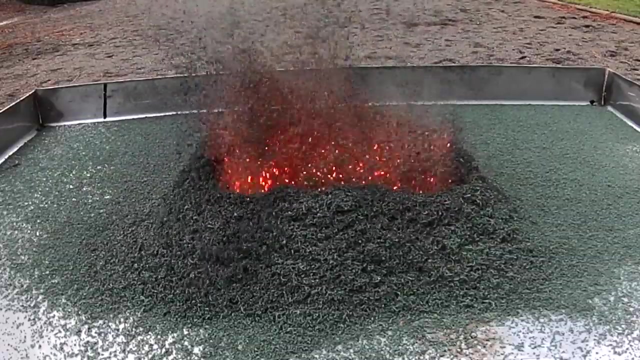 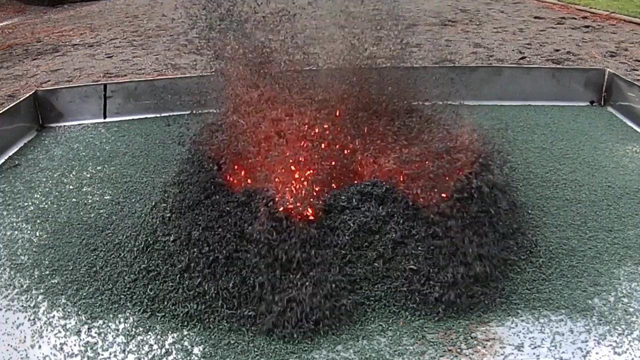 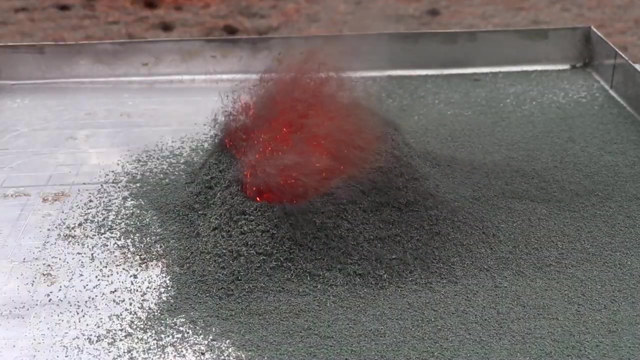 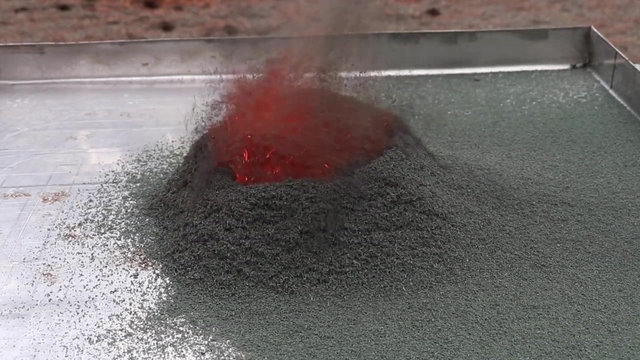 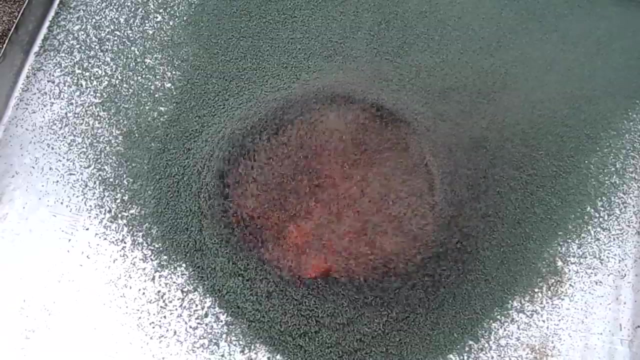 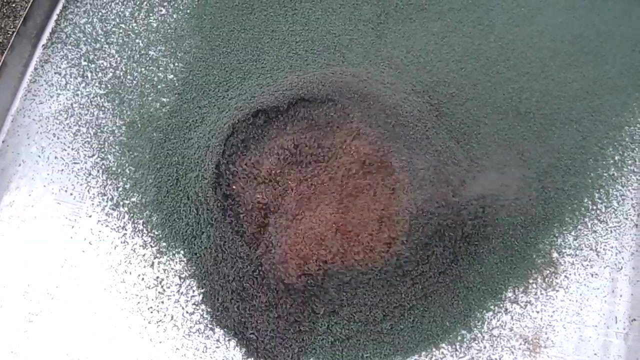 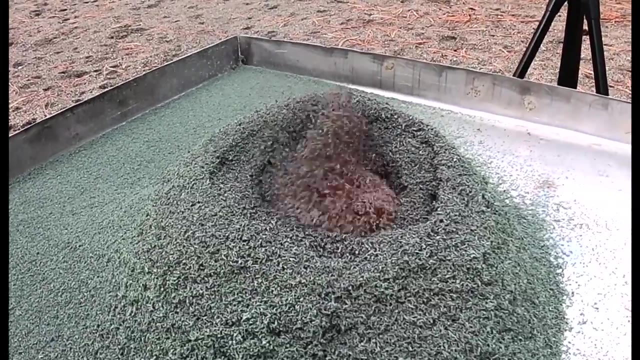 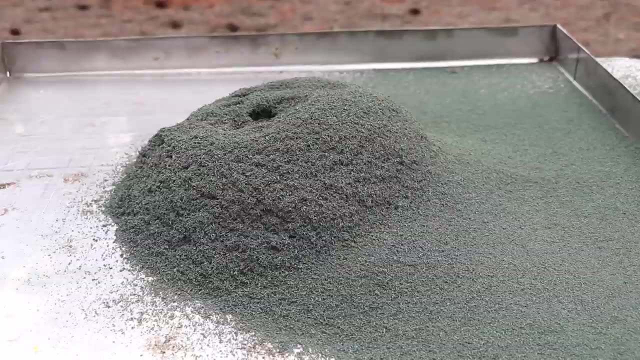 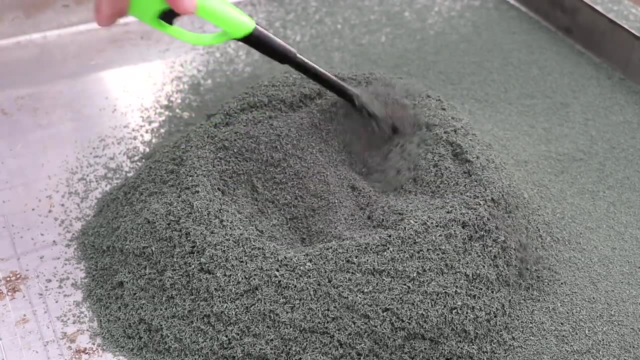 Let's do it again. Let's do it again. Wow, Are you crazy? Wow, That was crazy. Look at that. Oh, it's still hot. Let's see what is on the bottom there: Nothing, It just becomes this powder. 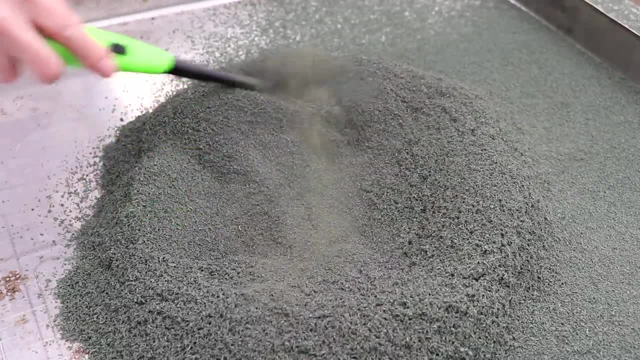 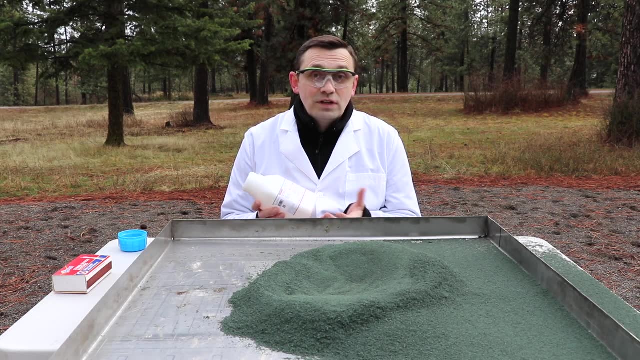 Well, thank you guys for watching. Let me know in the comments if you like this type of videos. I'm planning to make more videos like this. See you in the next one. Bye, I'll see you next time, Bye, Bye.